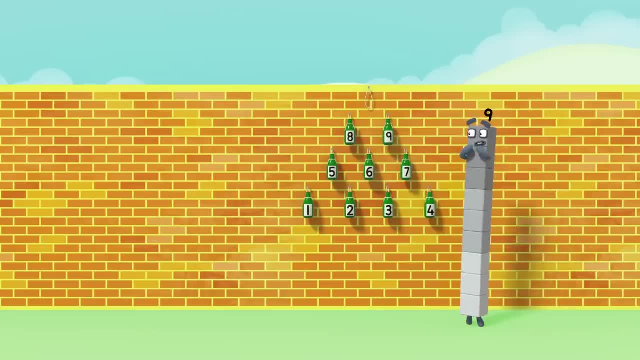 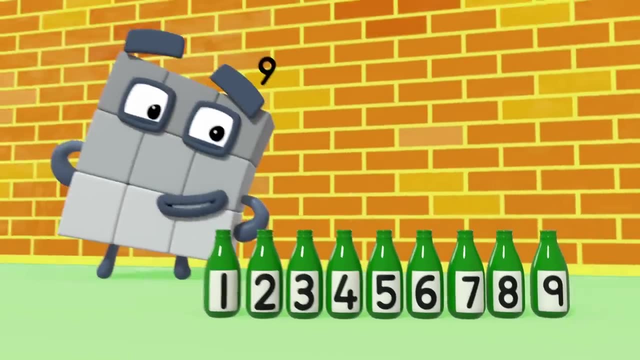 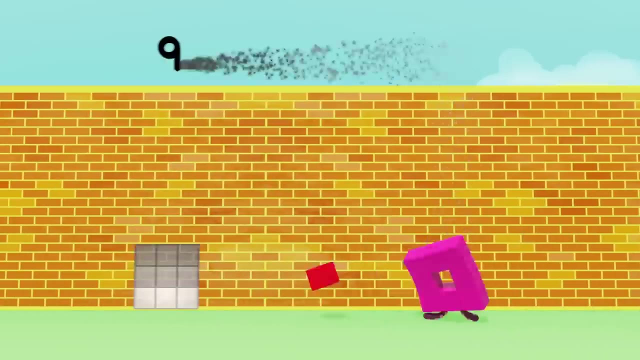 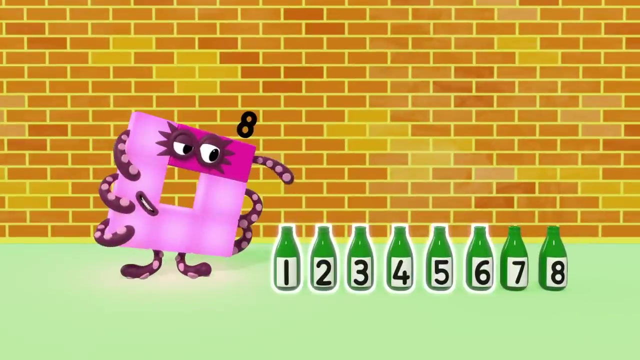 Nine green bottles hanging on the wall. Better move these nine before they fall. They're not safe up there. Nine green bottles safely on the floor. Nine green bottles safely on the floor, But if one green bottle becomes a dinosaur, There'll be one, two, three, four, five, six, seven, eight. 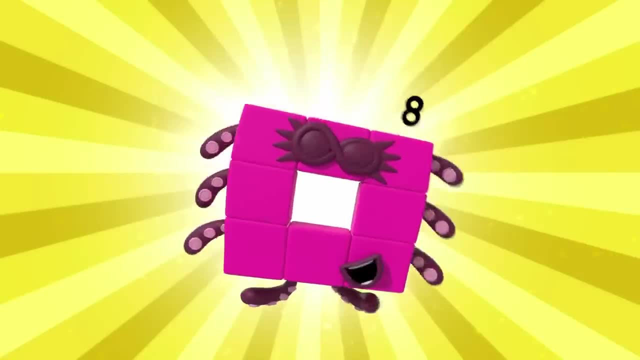 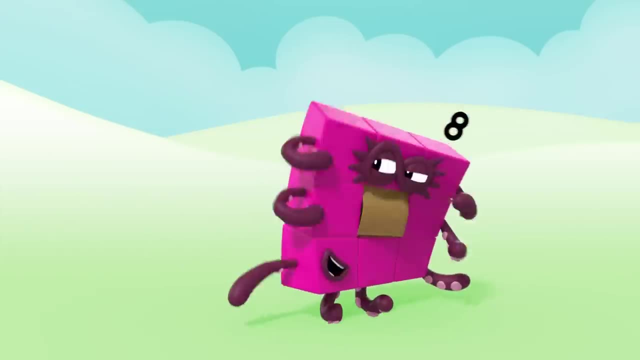 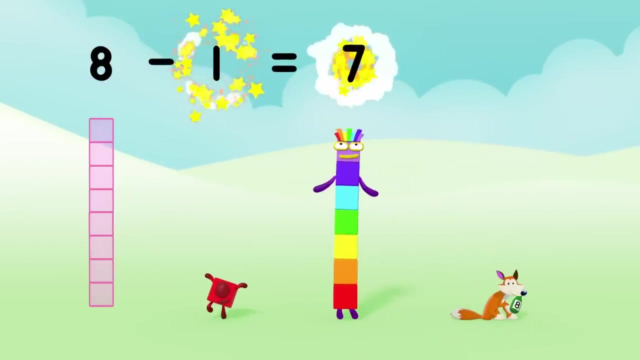 Eight green bottles not safe on the floor. Octoblock: hide One, two, three, four, five, six, seven, eight. hide Seven green bottles hiding in a box. But if one green bottle is stolen by a fox, 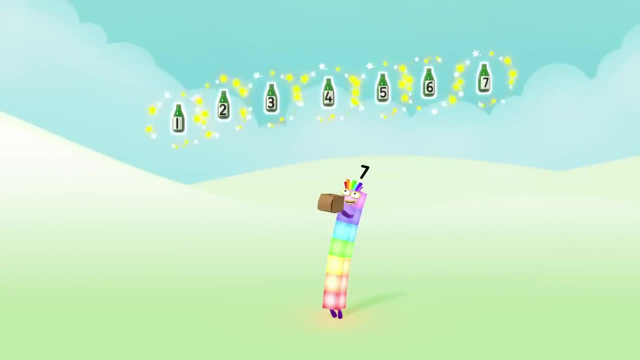 There'll be one, two, three, four, five, six, seven, Seven green bottles hiding in a box. That was lucky. Seven green bottles flying through the air. Seven green bottles flying through the air, But if one green bottle should wake a grizzly bear. 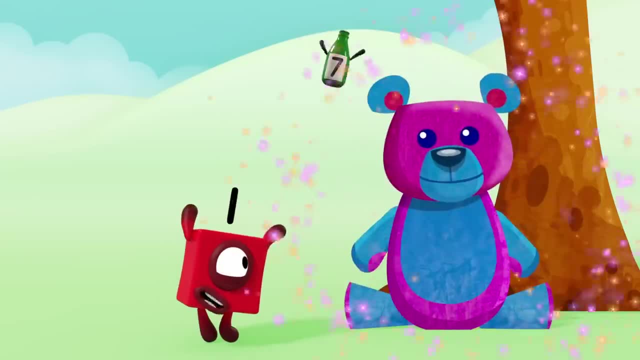 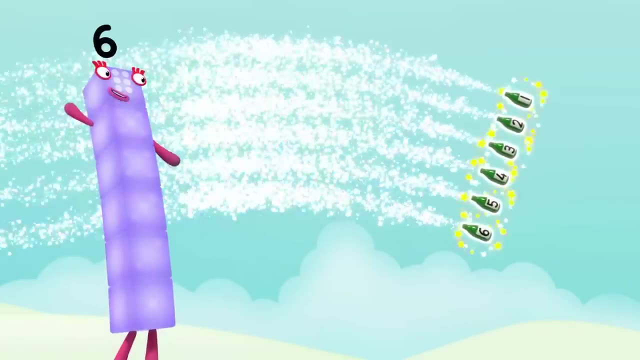 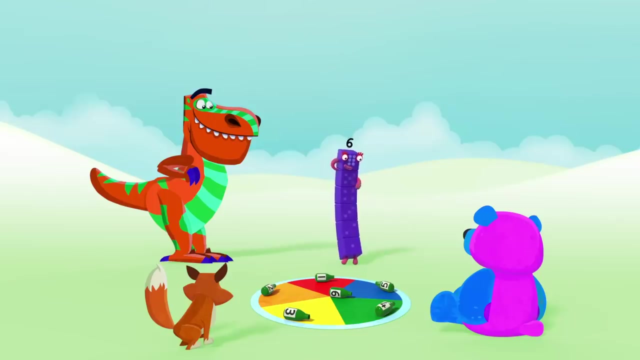 What I mean. hug a teddy bear. Phew, There'll be one, two, three, four, five, six, Six green bottles falling through the air. Six is my name. let's play a game, And this game goes like this: 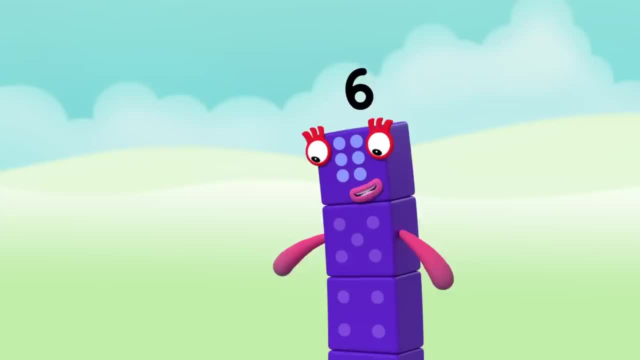 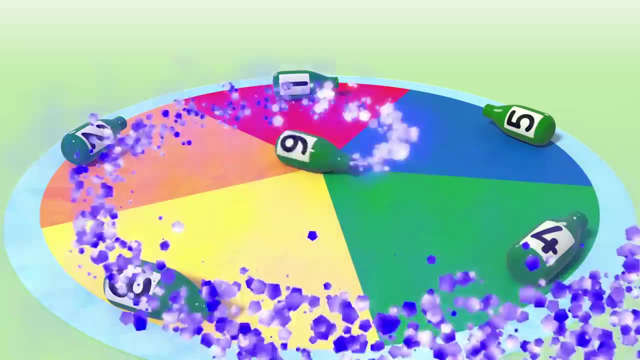 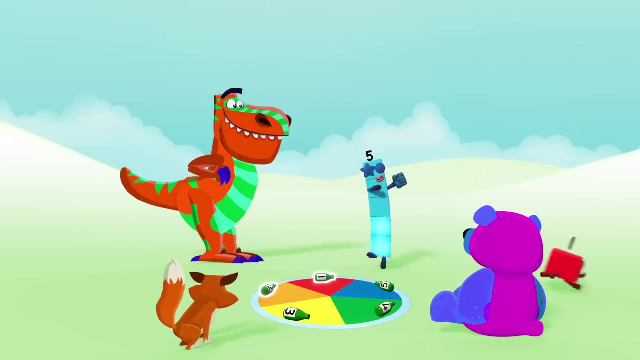 Six green bottles lying on the ground. Six green bottles lying on the ground, Six green bottles lying on the ground, And if one green bottle spins around, Whoa, You win. There'll be one, two, three, four, five, Five green bottles lying on the ground. 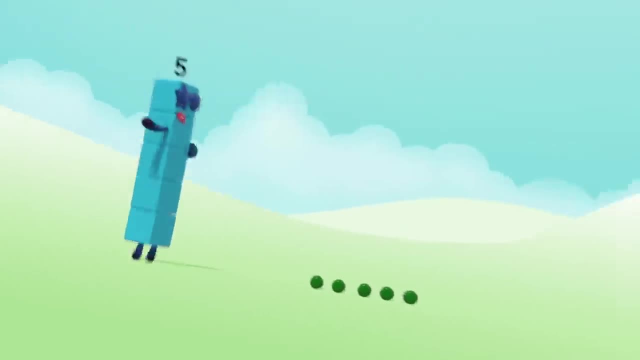 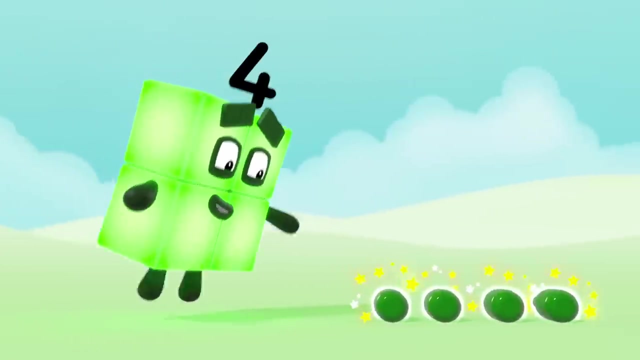 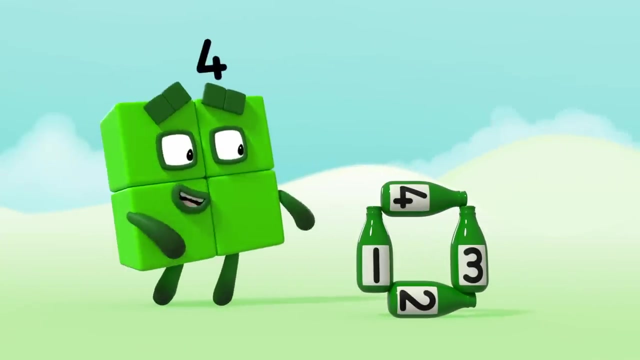 Five green bottles rolling down the hill. Five green bottles rolling down the hill, But if one green bottle should grow a daffodil, There'll be one, two, three, four, five green bottles Rolling down the hill, Four green bottles standing in a square. 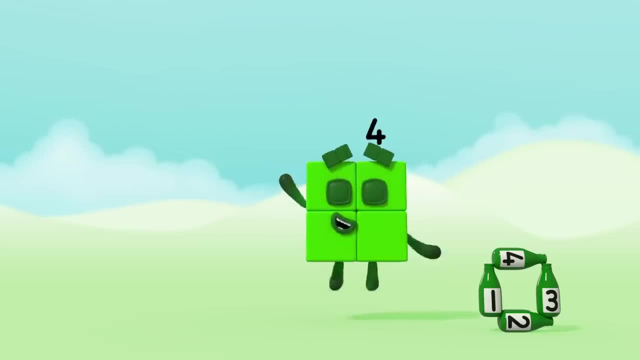 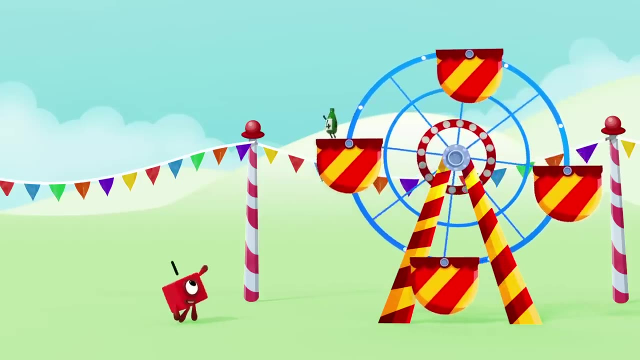 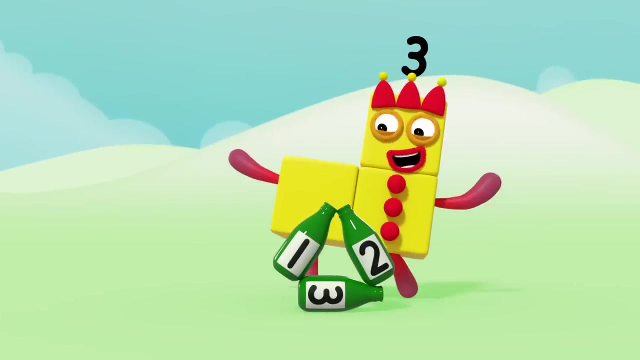 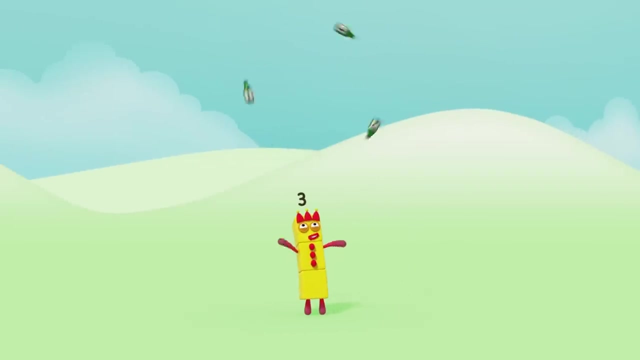 Four green bottles standing in a square, But if one green bottle should run to the bear, There'll be one, two, three, three green bottles Standing in a triangle. One, two, three, Three green bottles spinning in the sky. Three green bottles spinning in the sky. 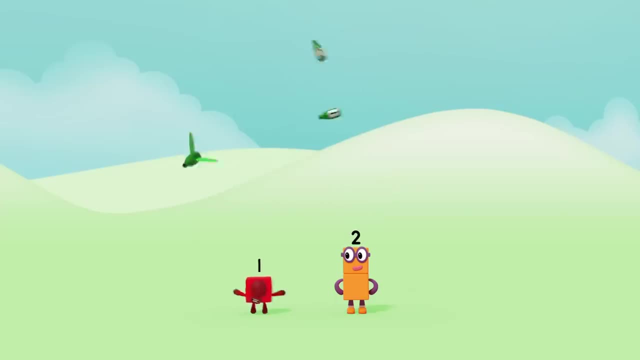 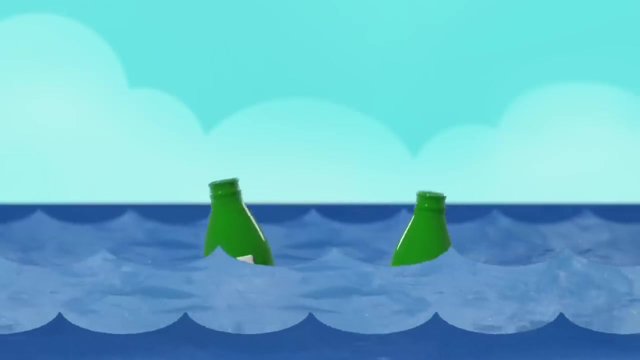 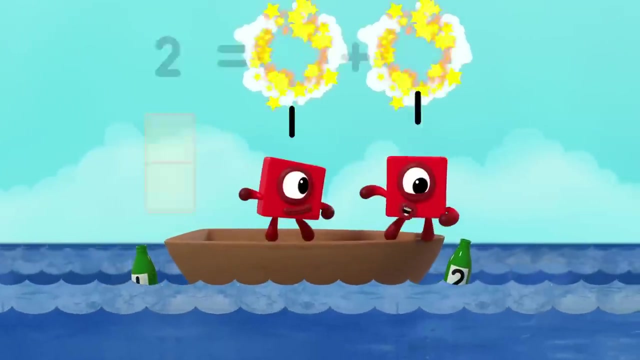 But if one green bottle should drop its wings and fly, There'll be one, two, three green bottles spinning in the sky. Come back, Two green bottles floating out to sea, Two green bottles floating out to sea. But if one green bottle should learn to water-ski? 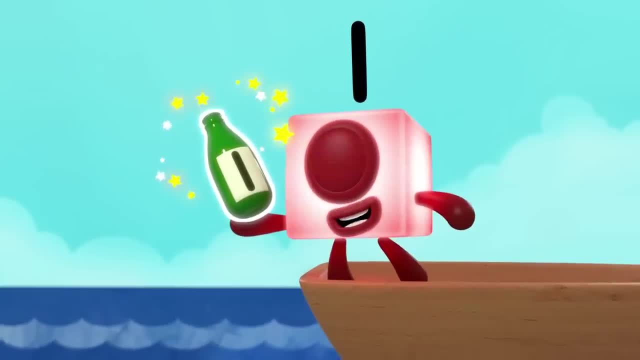 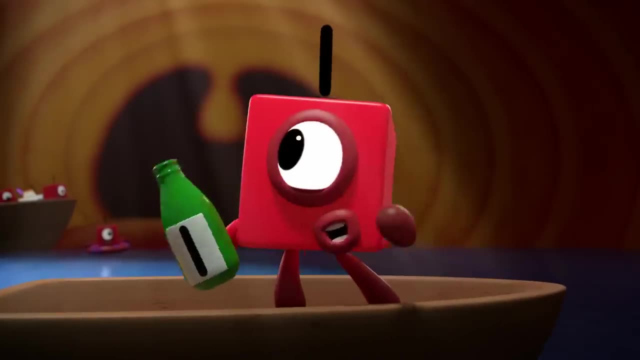 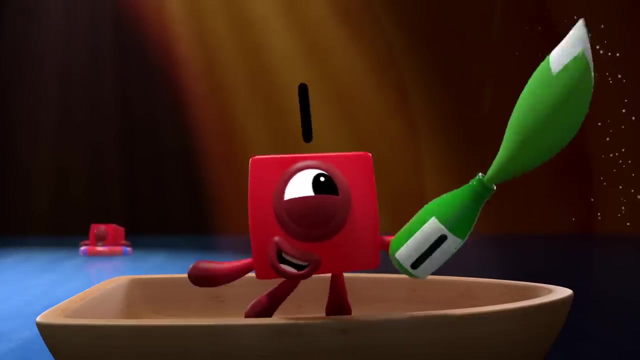 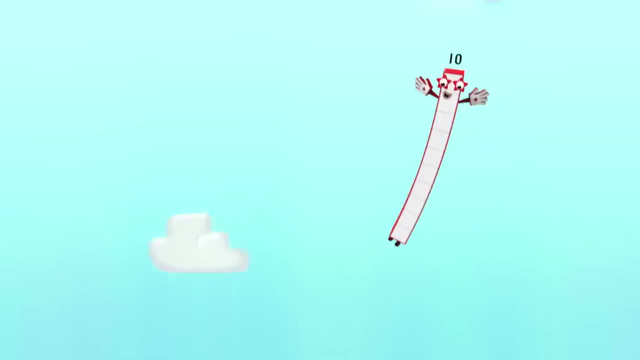 There'll be one. One green bottle floating out to sea, One green bottle swallowed by a whale. One green bottle swallowed by a whale. But if that green bottle should grow a tickly tail, There'll be no green bottle swallowed by a whale. Ten green bottles hanging on a wall. 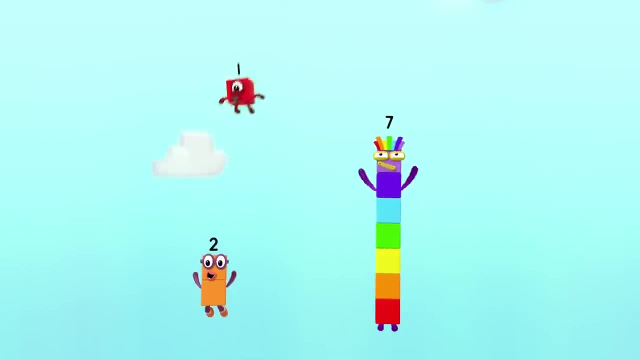 Slightly on the floor, Hiding in a box, Flying through the air, Lying on the ground, Ten green bottles rolling down a hill, Standing in a square, Spinning in the sky, Floating out to sea Swallowed by a whale. But if one green bottle should accidentally fall, 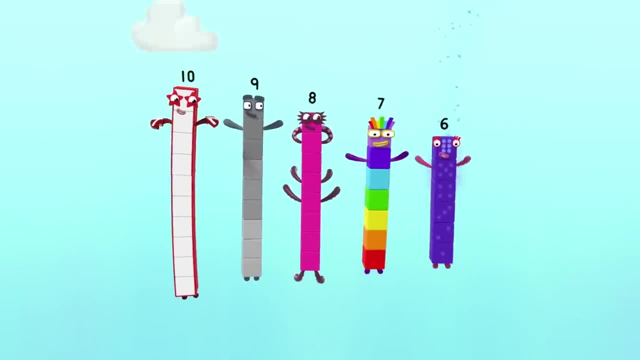 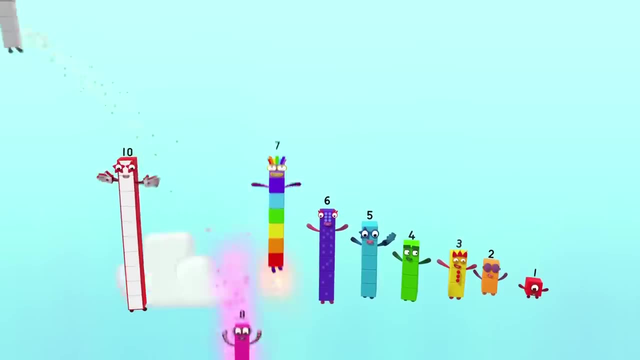 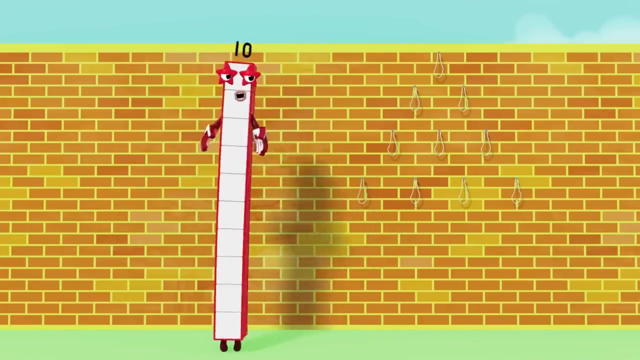 Become a dinosaur. Wake a grizzly bear, Spin around up a hill, Flap its wings and fly, Learn to water-ski. Grow a tickly tail. There'll be nine, eight, seven, six, five, four, three, two, one. No green bottles hanging on the wall. 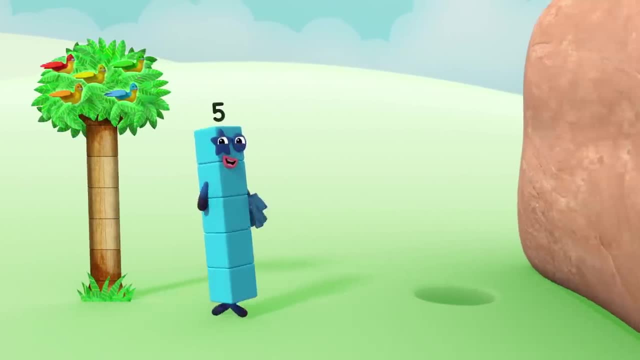 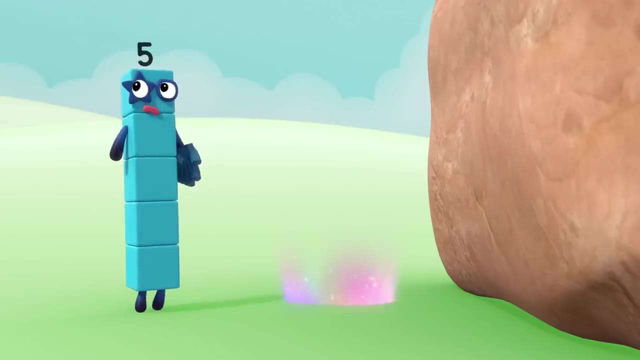 One, two, three, four, five. What a wonderful day to be alive. A giant rock in front of me. How can I get where I need to be? What is that silly sucking sound? Oh, look, a hole so big and round. 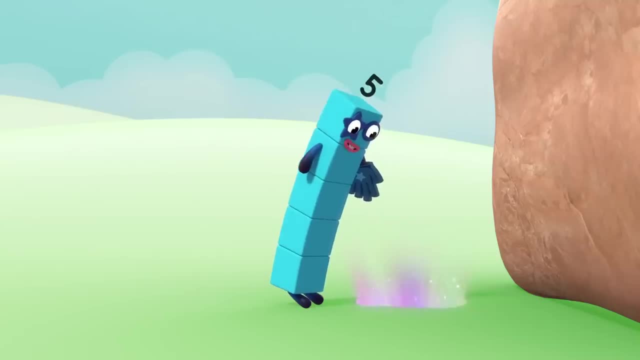 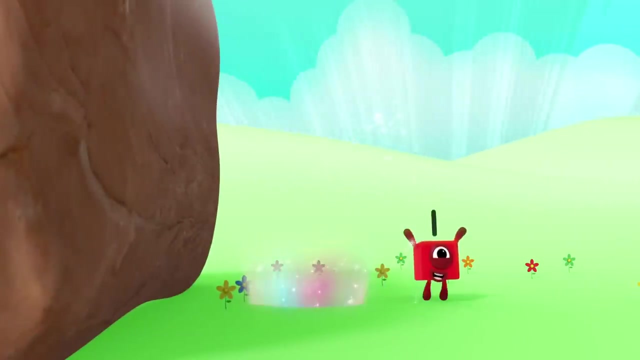 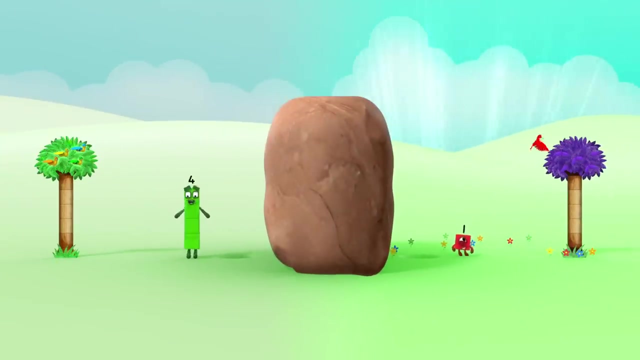 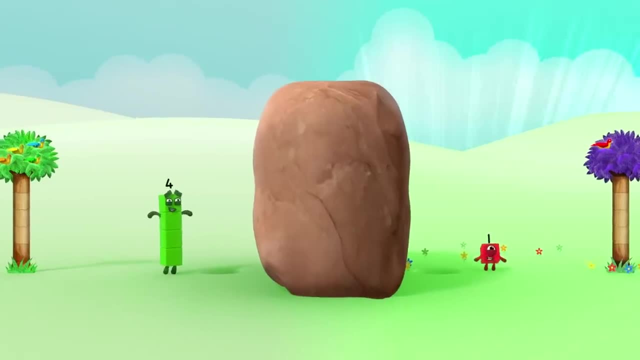 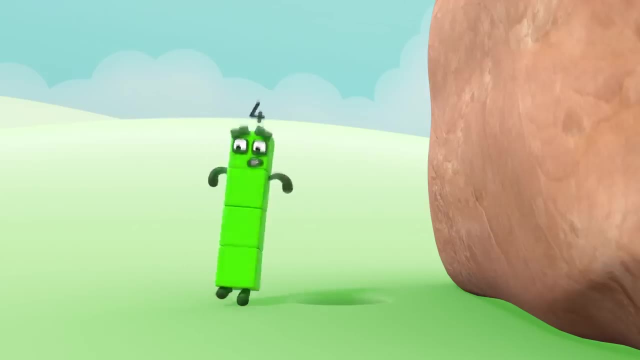 I am one Here. I am. What a wonderful day to be alive. But where, oh, where, oh, where is five? Five is gone. where did she go? Is she alright? I do not know. Is she here, Is she there? 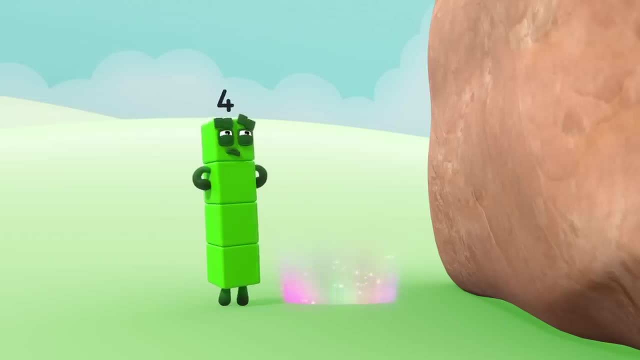 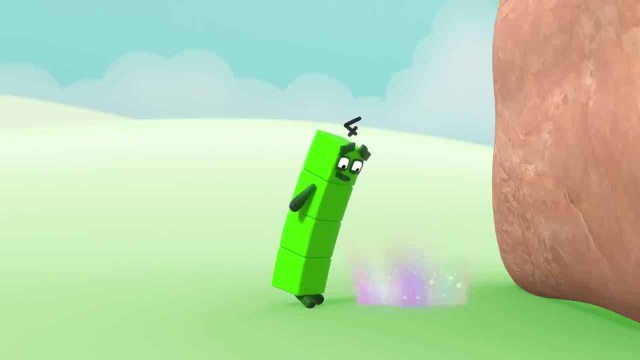 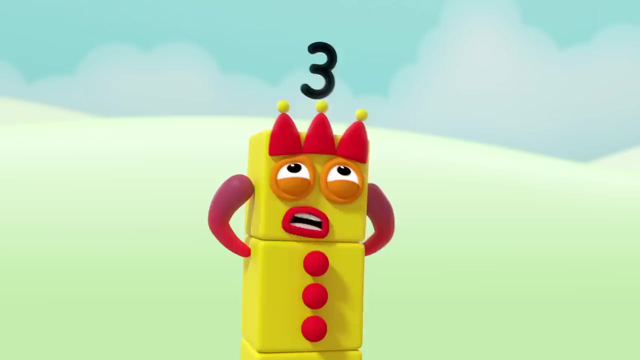 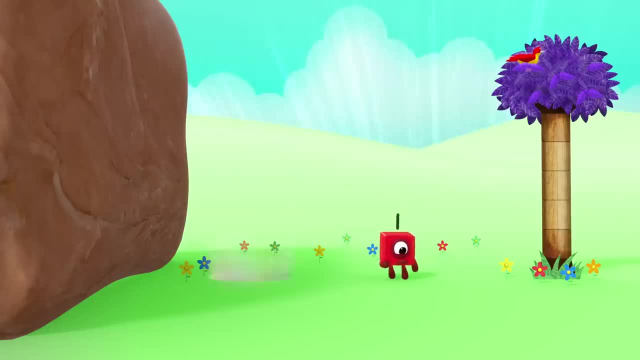 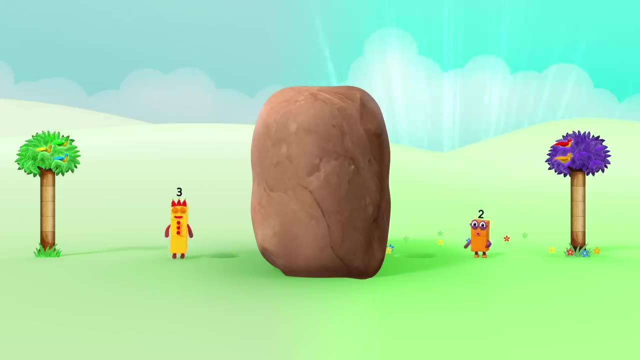 My head fell off. Where did it go? I am one. That was fun. I am one, That was fun. Now I am three, and here I am. Now I am two and here I am. What a wonderful day to be alive. But where, oh, where, oh, where is five? 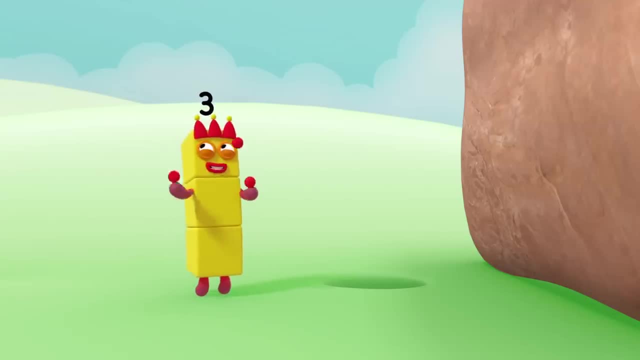 I was five, then four, then three. Someone has played a trick on me. I do not mind at all. you see, Three is who I want to be. What is that silly sucking sound? A giant hole so big and round. Why is it there? I do not know. 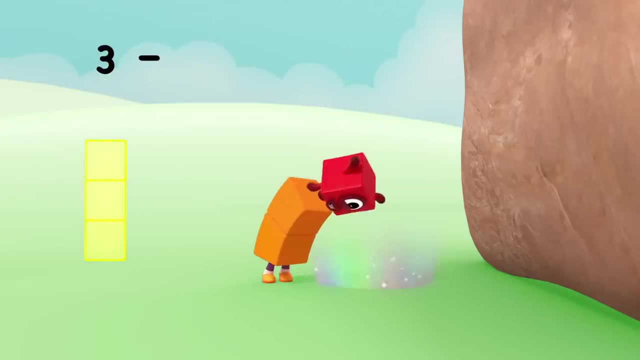 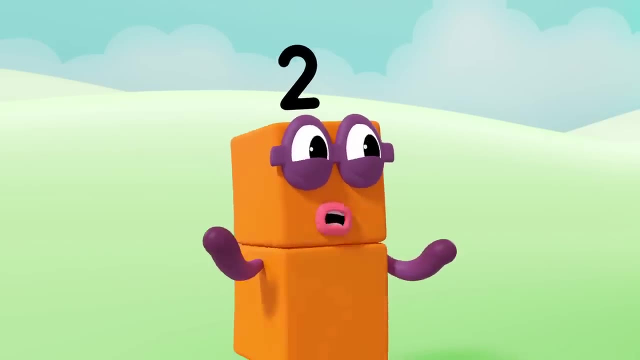 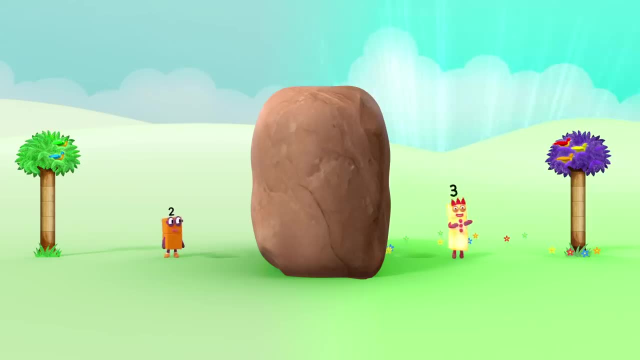 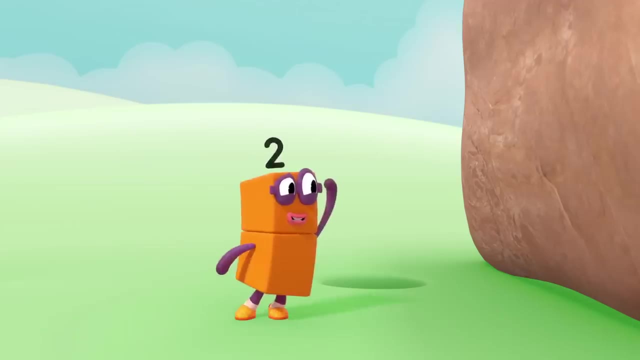 What a wonderful day to be alive. But where, oh where, oh, where, is five? I wonder where the ones will go. I think I've got it now. I know Every time we get one smaller, Someone else is getting taller. Three minus one equals two. 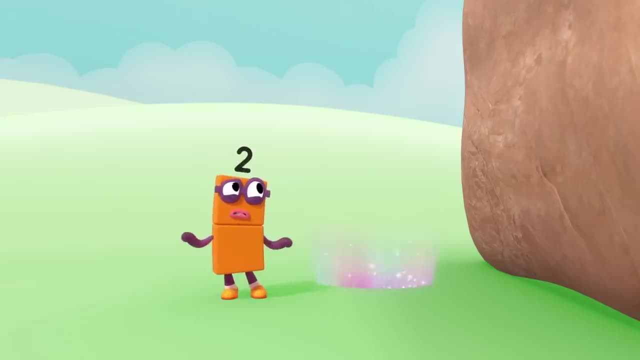 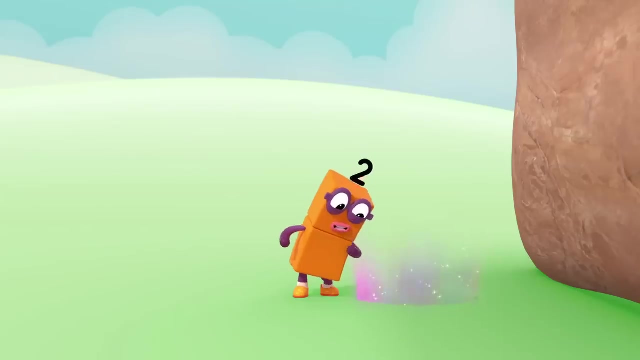 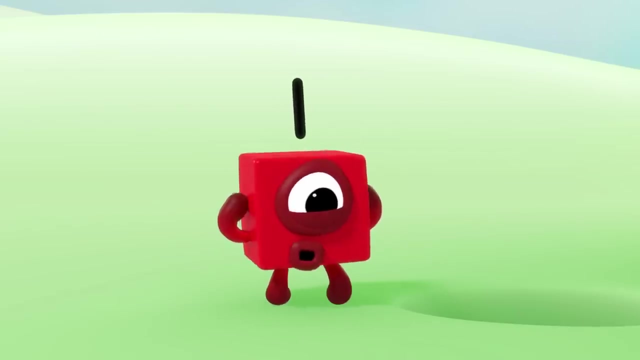 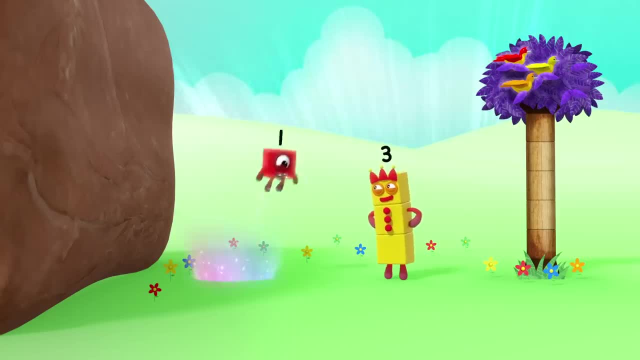 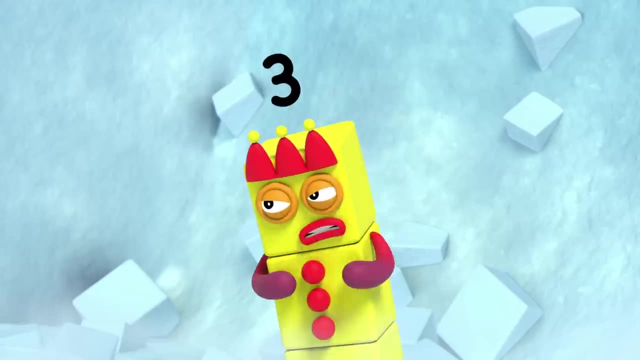 I am one. That was fun. Nine, Oh no, Where are you? It was me, I was nine And Big Charlie was a little better, But where is the whole team? How many, I don't know. I had my eyes shut. 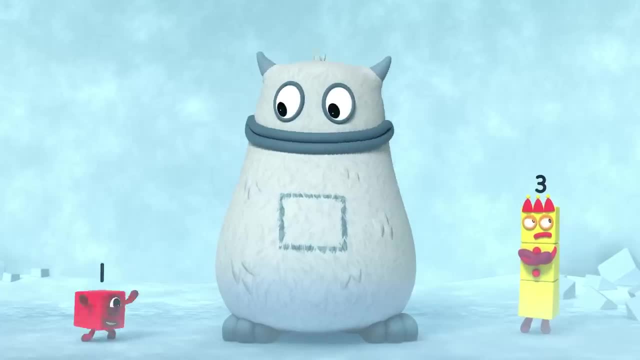 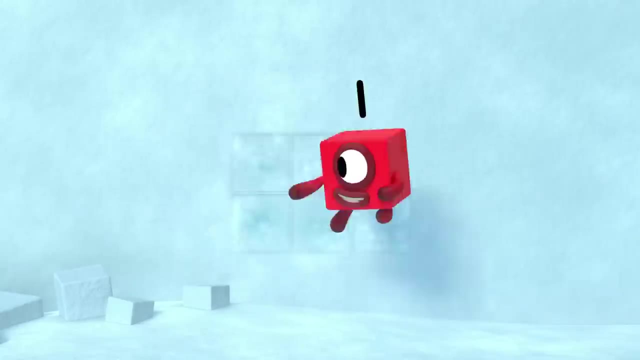 Oh I know, Here goes One, two, three, four, five, six, seven, eight, nine. So Nine was here. Then some of his blocks were taken away and that left you three, which means Nine minus Young. 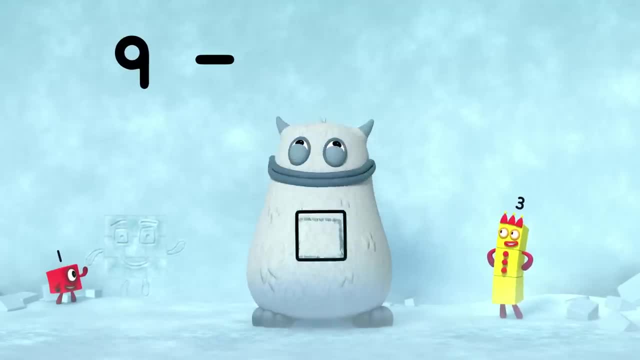 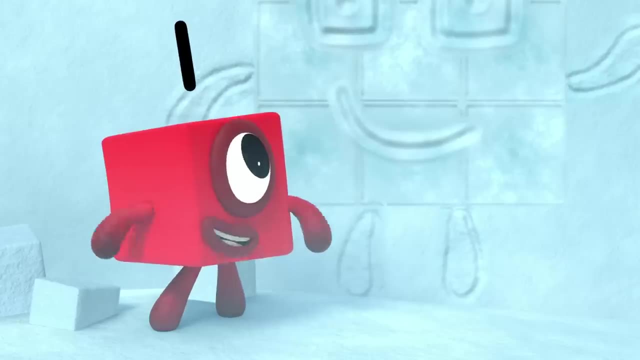 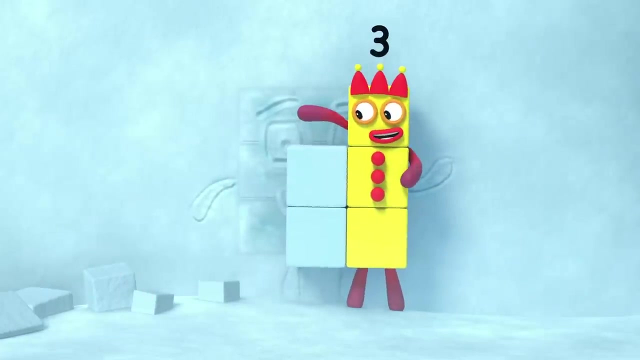 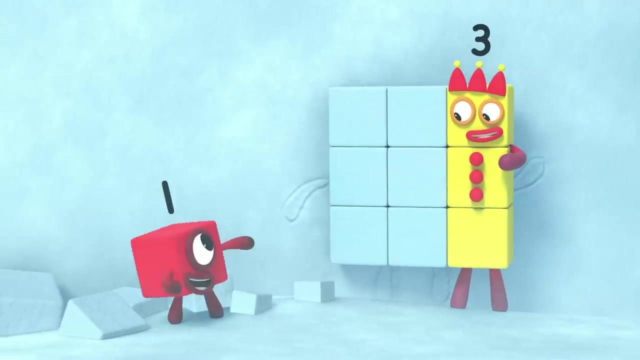 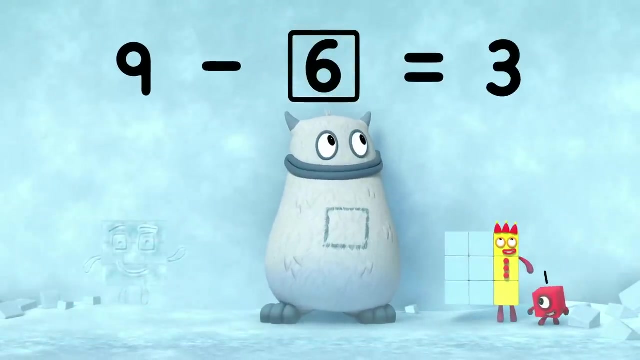 equals three. So what's missing? Hmm, Come over here. three, Hey, That's one, two, three, four, five, six There. So that's what's missing. Nine minus six equals three, And six is in your tum. 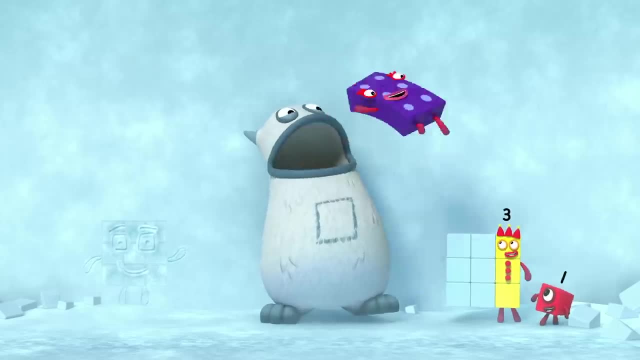 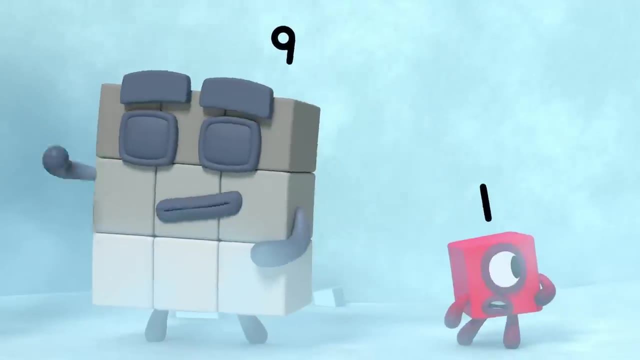 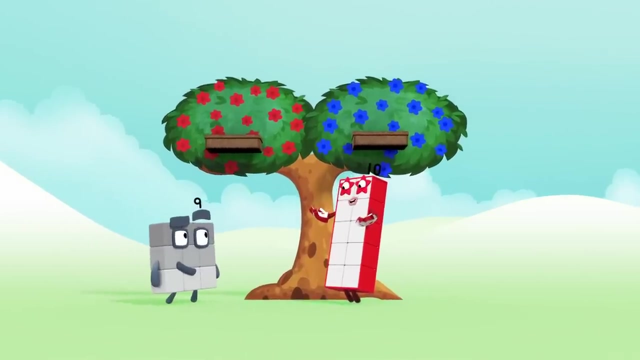 Yum, yum. Well done, Hooray. It's good to be back. Where are the others? Off to Black Sledge. Fancy a game of throwing twos. You be reds, I'll be blues. Sounds like fun. 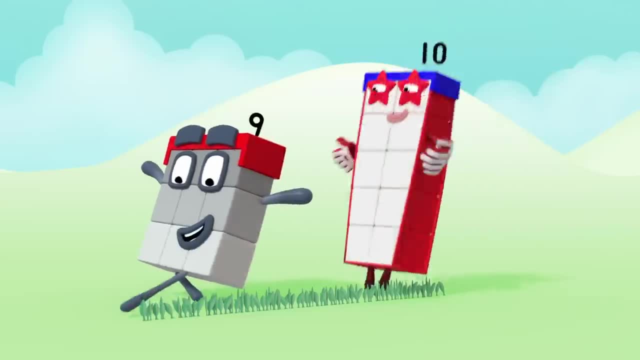 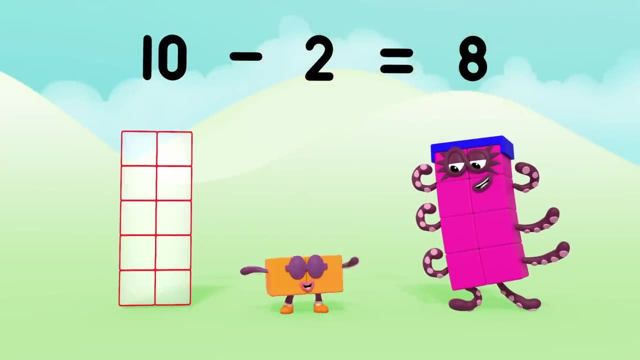 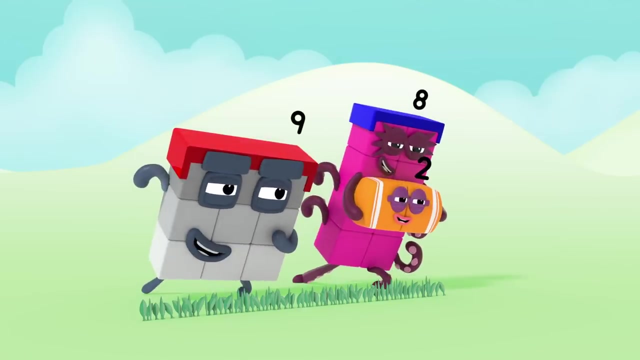 I'll draw a line. I'm bigger so I'll start. Ten minus two equals eight. Game on Ready go Off to block play. One, two, three, four, five, six, seven, eight play. 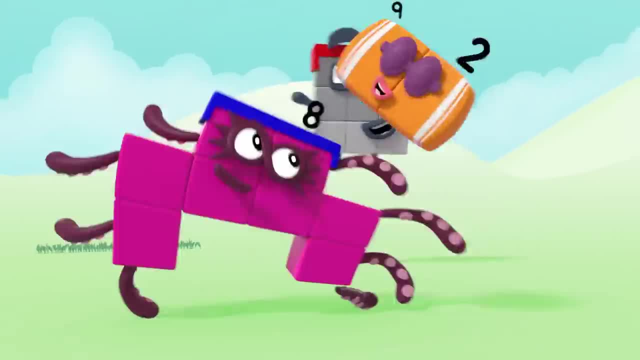 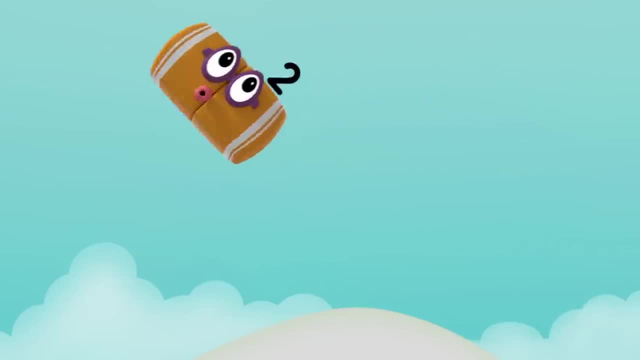 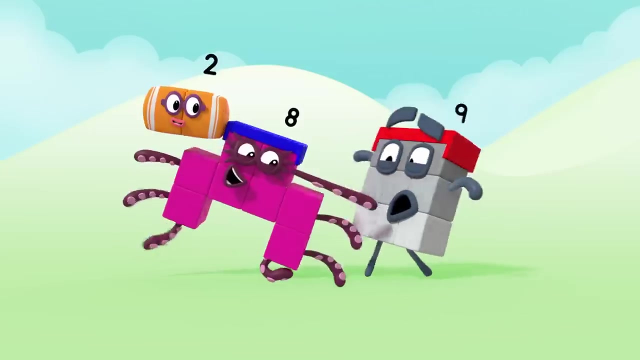 He's on the left And now the right. He's on my head And now he's on mine. Oh, Now out of sight. Woo-hoo. Up high, down low, Too slow, Achoo Whee. 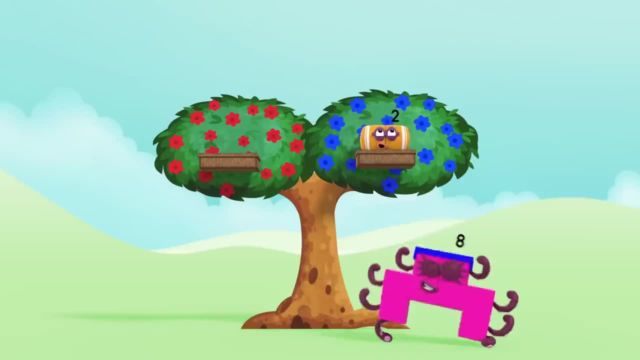 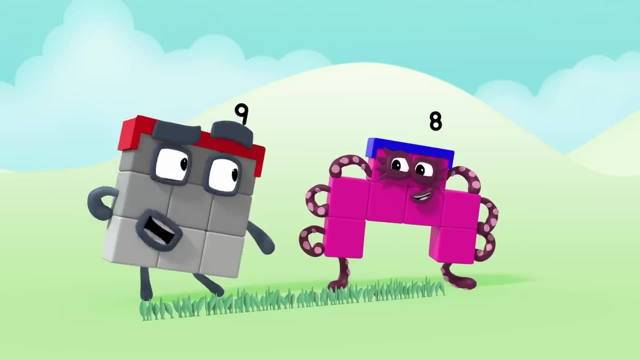 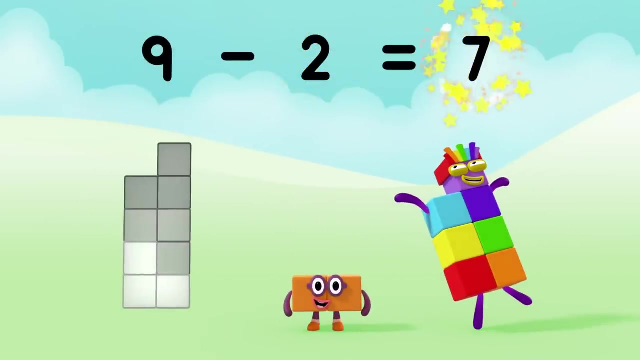 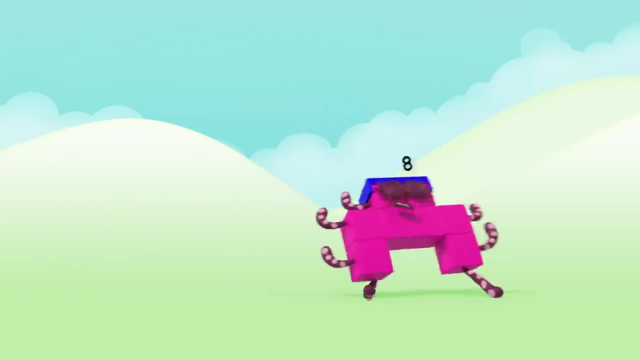 Off to block jump. Woo-hoo. Score Two points to blues. I'm bigger now, So it's my turn. Nine minus two equals seven. Ready go, Oh, Oh, Uh, Whee, Woo-hoo. 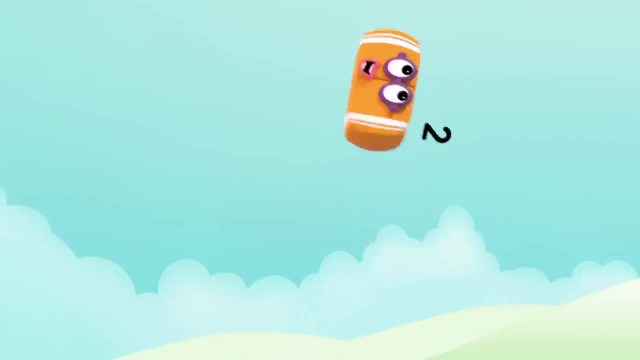 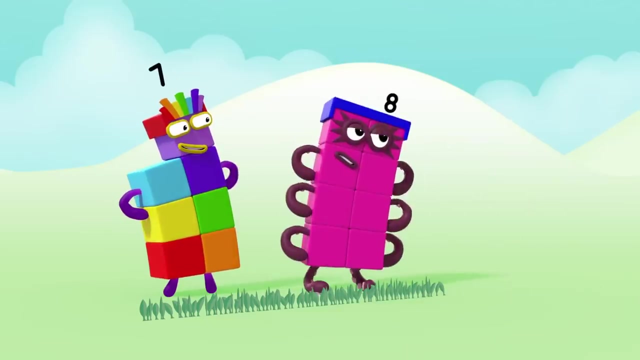 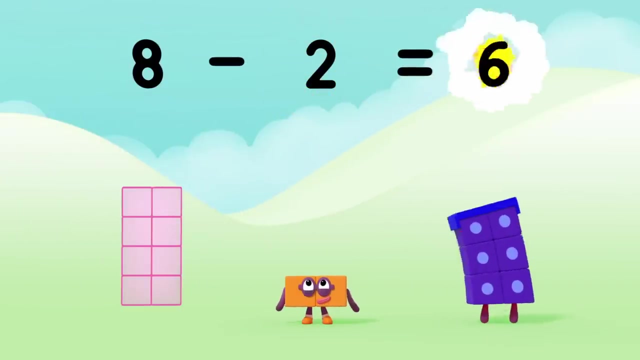 Woo-hoo, Oh, Oh Whee. Two points each Beginner's luck. You're bigger now. You're bigger, You start. Eight minus two equals six. Whee, Whee, Whee, Whee. 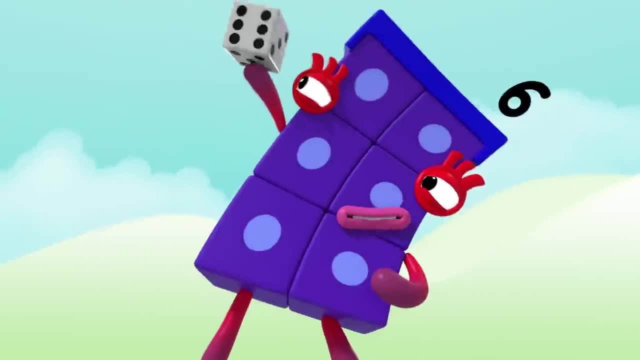 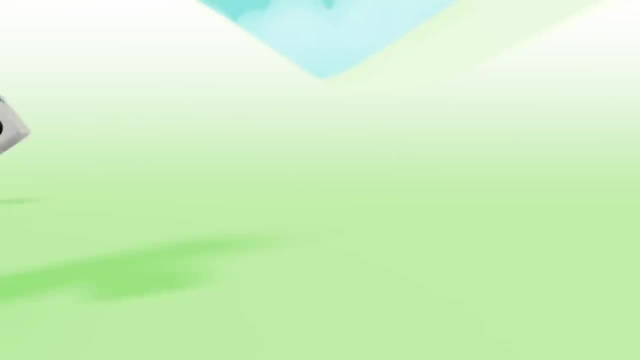 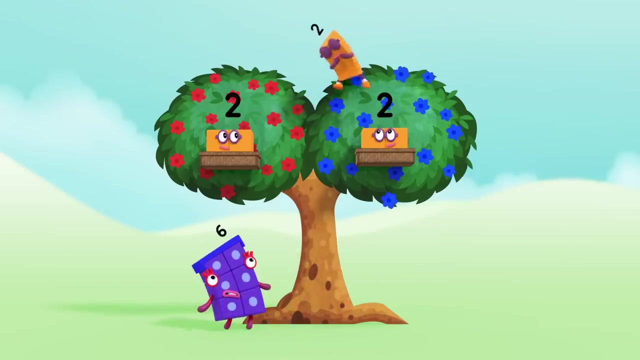 Whee, This game is nice. Let's roll the dice. When it leaves my hand, how will it land? Um on six? Oh, Oh, Oh, Oh, Lucky me, Lucky me. Woo-hoo, Penalty, unfair distraction, which means four-two. 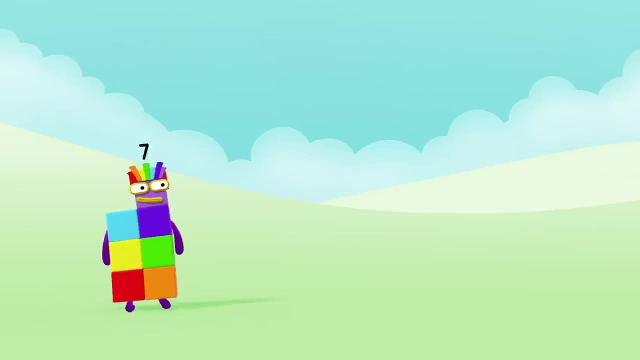 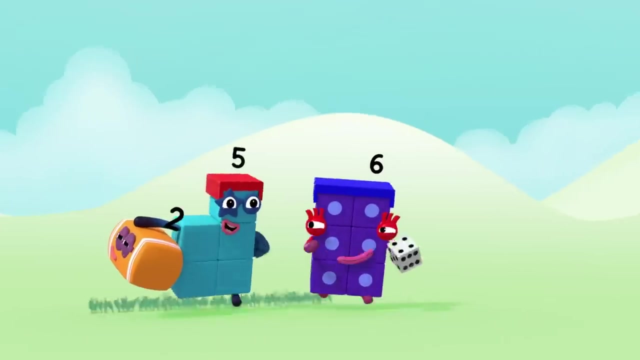 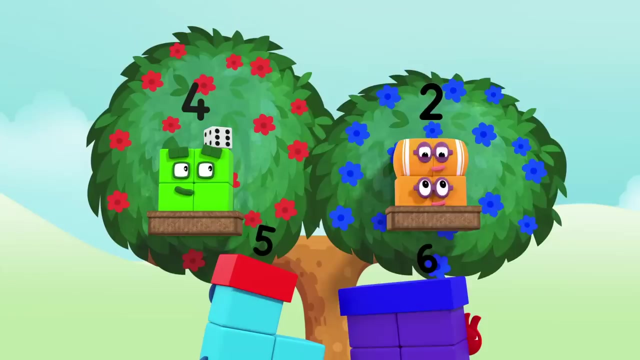 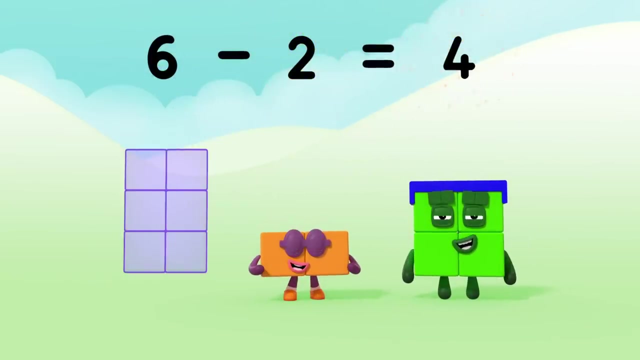 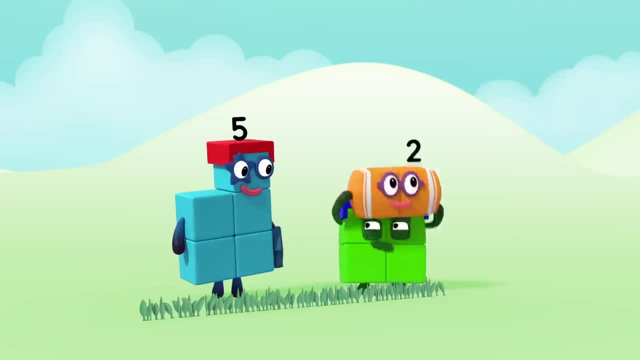 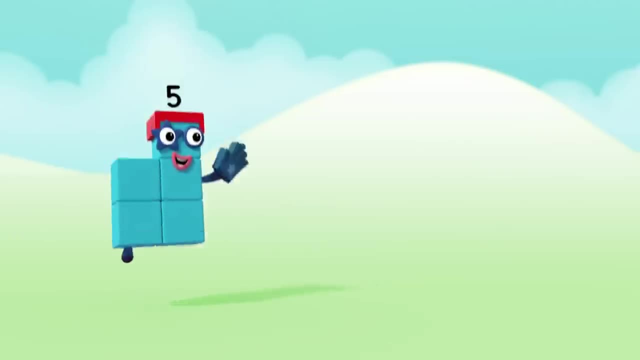 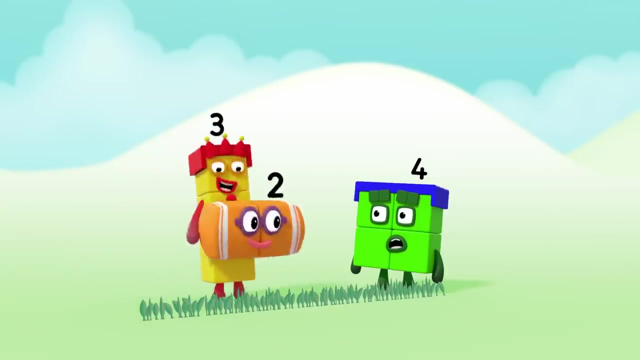 Oh, Ooh, Oh, Ohh, Ohhh, Whee, Whee, No, What's going on? What's going on What? I thought we were in some sort of truce Espa, What, What. 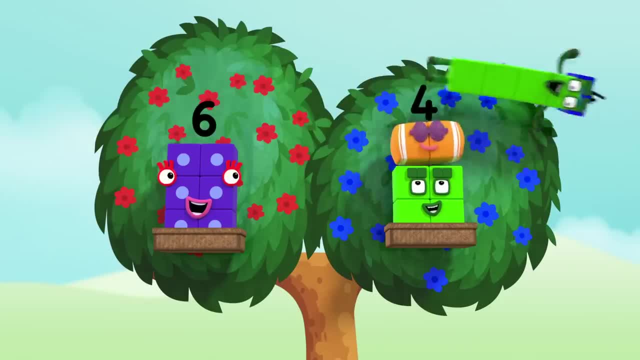 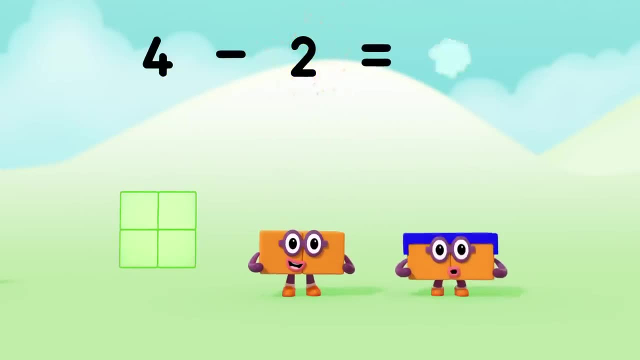 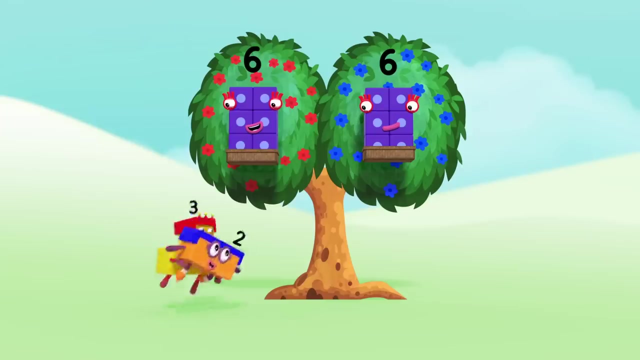 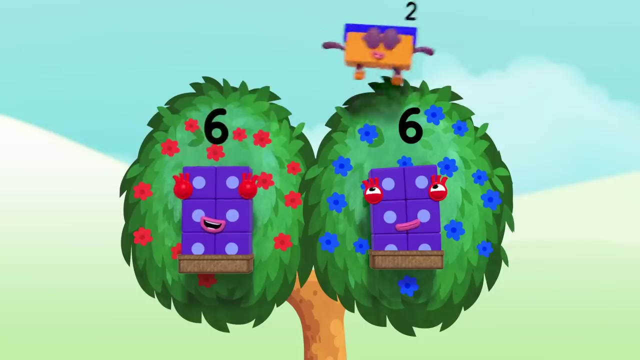 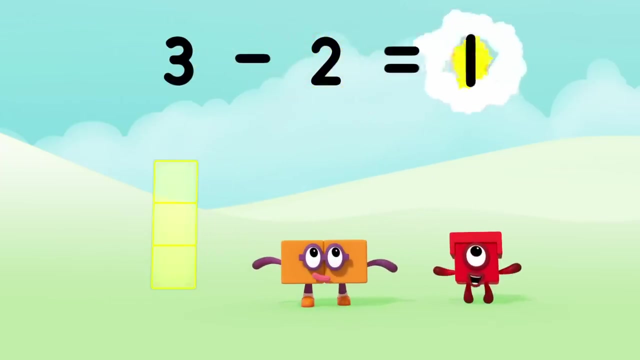 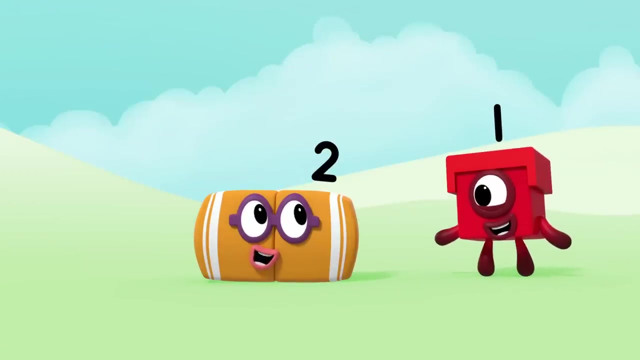 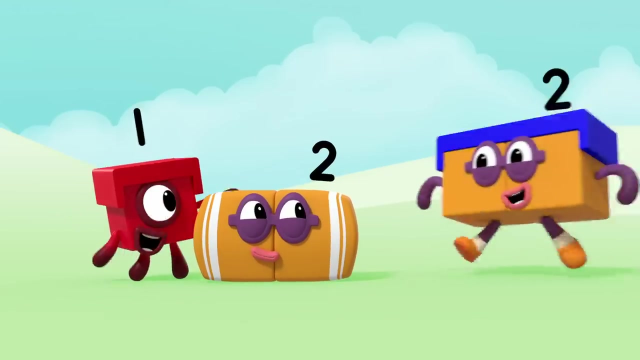 Six points each. Four minus two equals two. Hey, not me. Penalty round two, Oh Six Eight. Three minus two equals one. Final round. Ready go, Oh bother. Let me lend a hand or two, Thanks two. 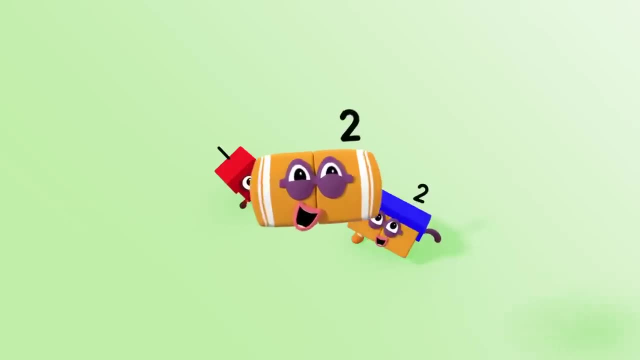 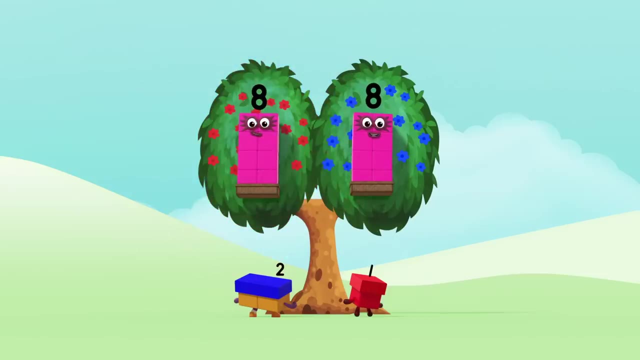 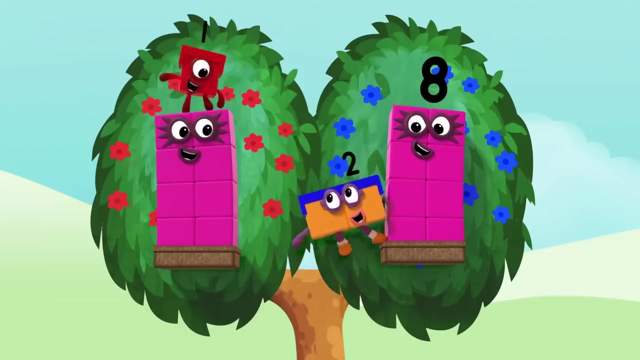 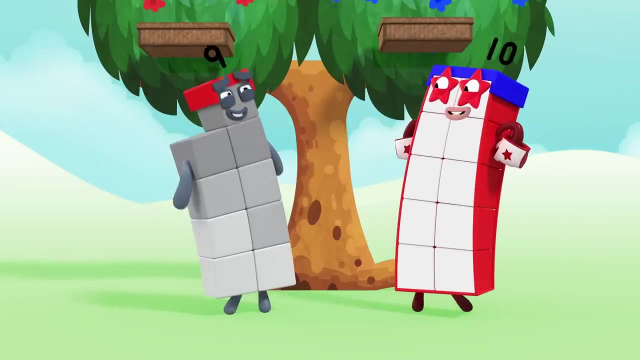 Up there please. One, two, Yay There, Hang on. Eight points each. It's a draw. Woo, That was fun. Same time tomorrow. Game on. Game on. Welcome to the Numbah Block Rally. 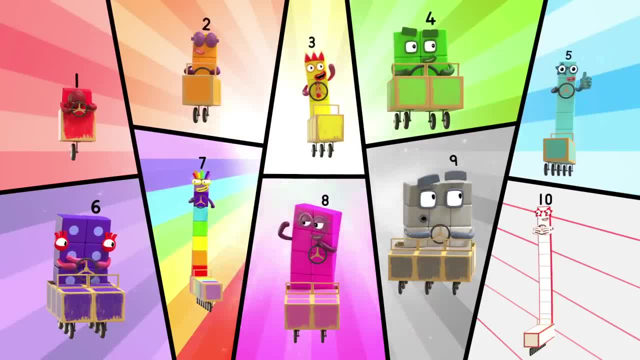 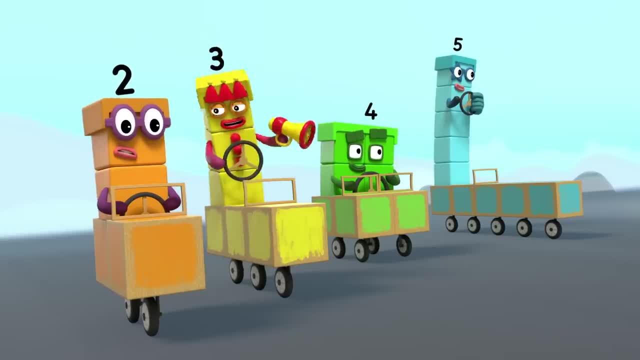 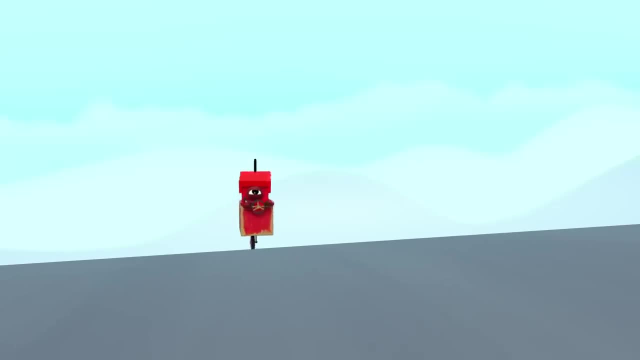 Ten riders, ten pedal-powered cars And only one can lift the trophy. So let's go over to the start line. Everybody ready? Hey wait, Has anybody seen one Coming? Pedal pedal, pedal, pedal, pedal pedal. 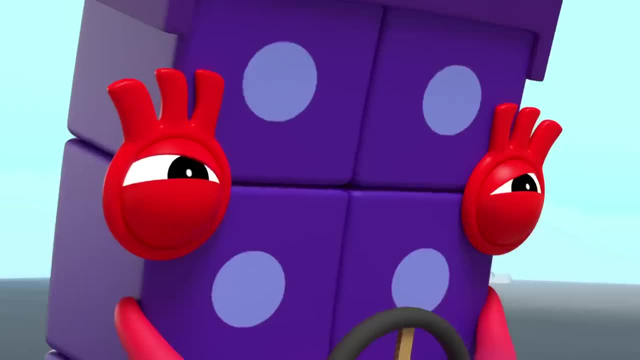 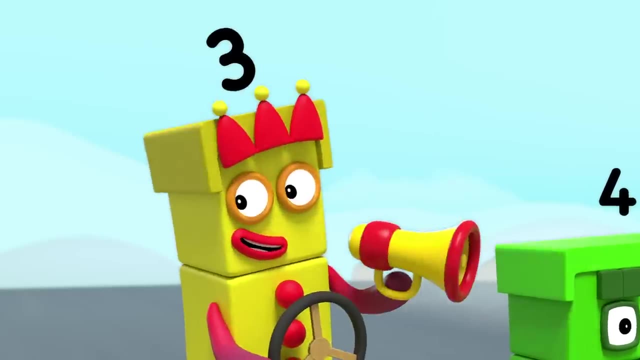 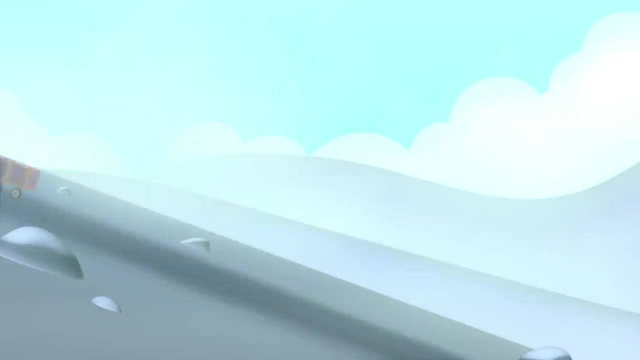 Let's go Vroom. Hope you're ready to play with the high rollers. I'm ready. Steady, Go, Go, Go, Go for it. Righty prisons on you kids. Nice car, eh, Yay. 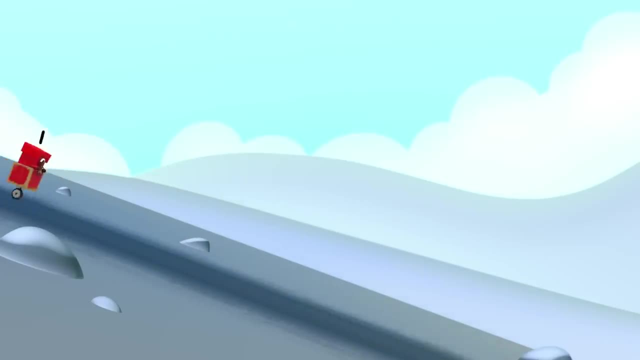 We won. I love it. That was fun. I love it. I love it too. A-a-ha, I say: go, I'm a pro Moose, I'll run the test even faster than that car Yay. 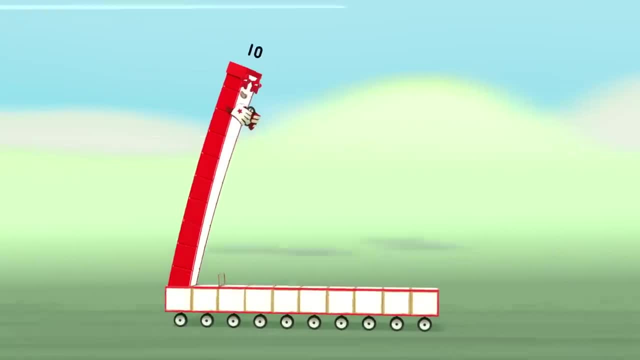 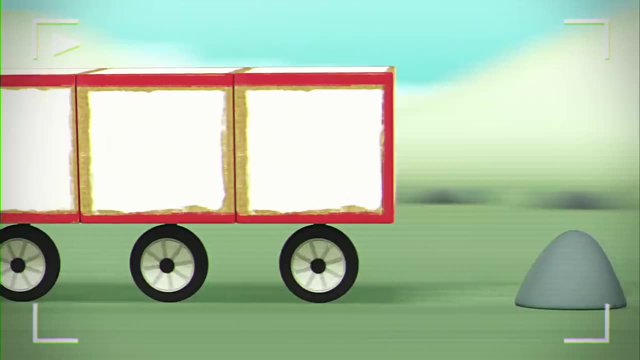 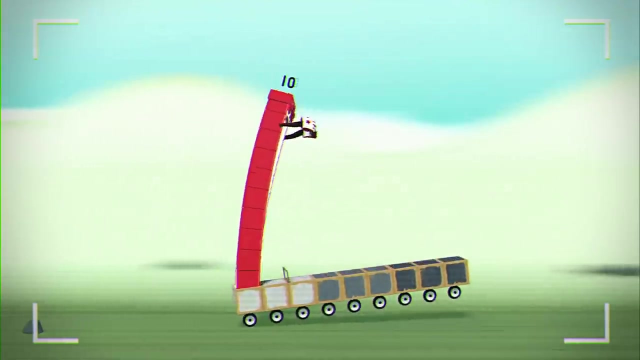 Hooray Ten is in the lead With ten wheels. she seems unbeatable. But wait, She's lost a wheel. Let's see that again in slow motion. Yay, What Ten wheels minus one wheel equals nine wheels left. 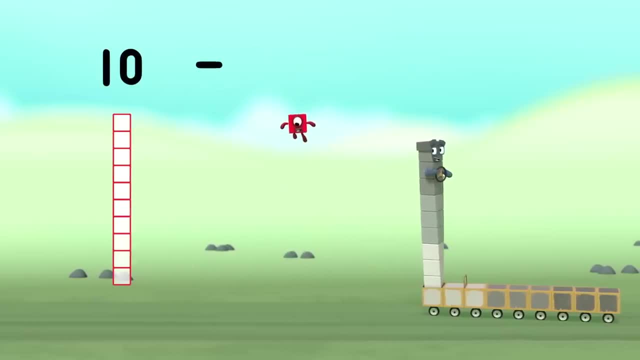 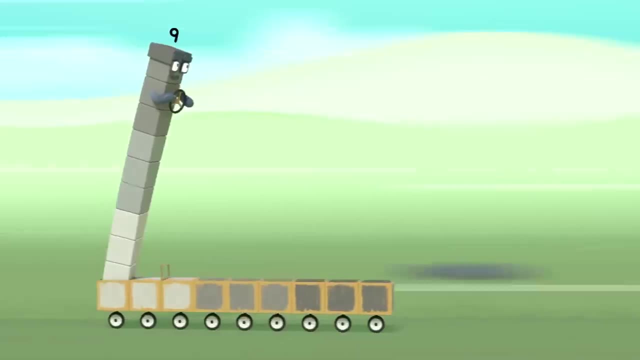 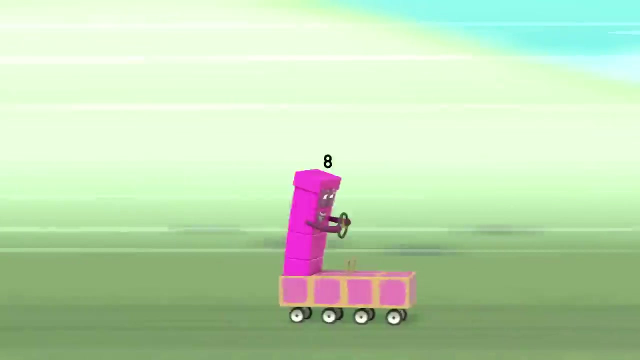 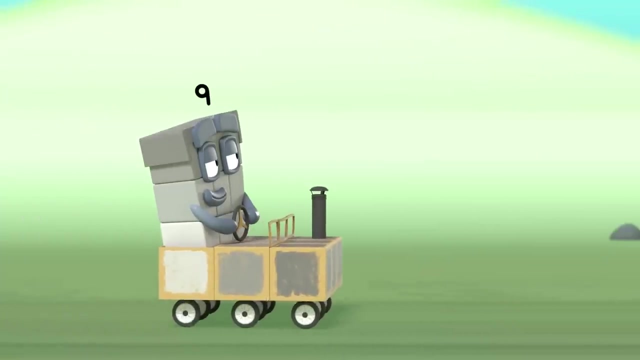 Ten minus one equals nine. Hey go, nine. Ten is out of the race as nine takes a surprise lead. Nice day for it. And what makes it really surprising is that nine's in last place too. Well, next to last, keep pedalling, Ron. 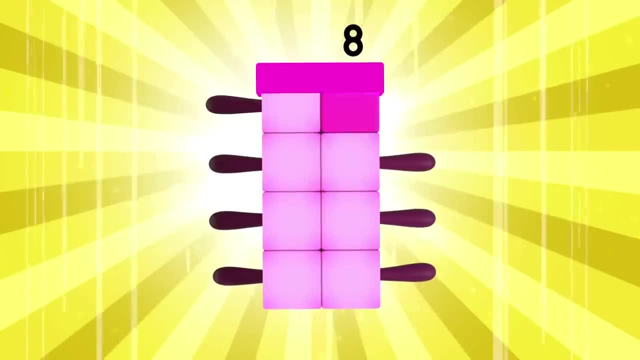 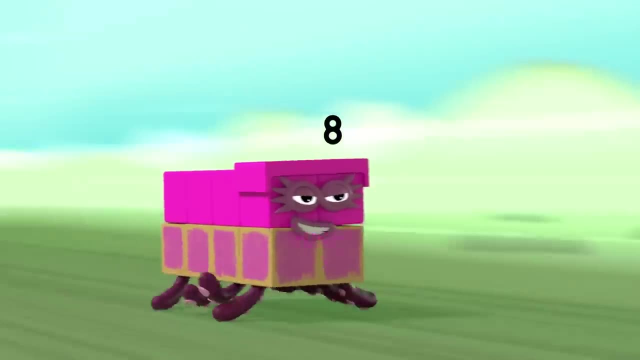 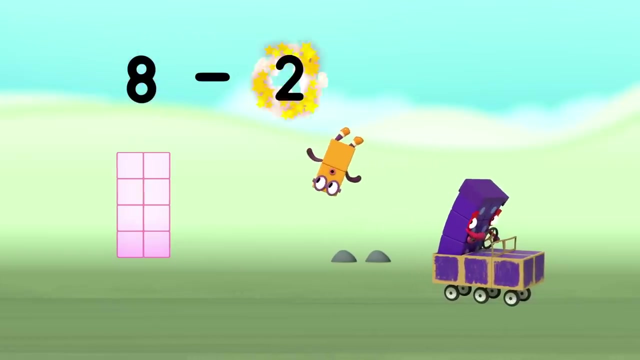 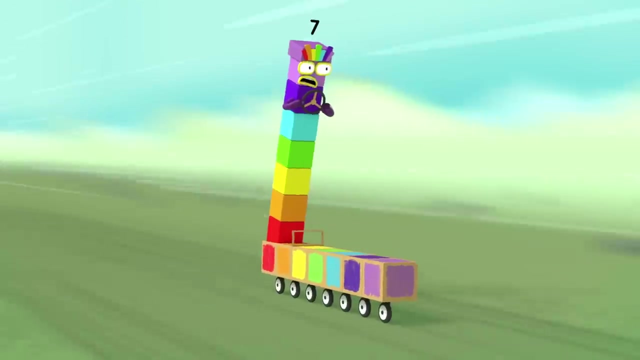 Octoblock race One, two, three, four, five, six, seven, eight race. It's in trouble. Those two squabblocks are about to go. Eight Minus two Equals six, Look out. 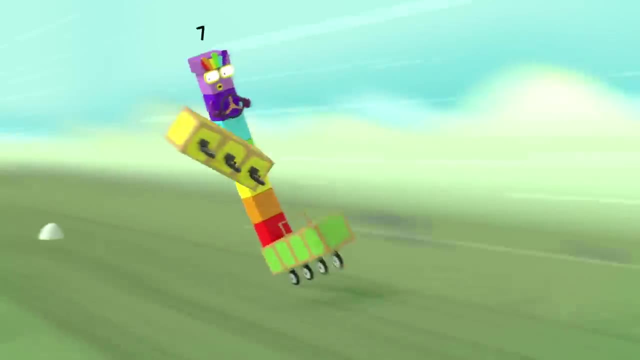 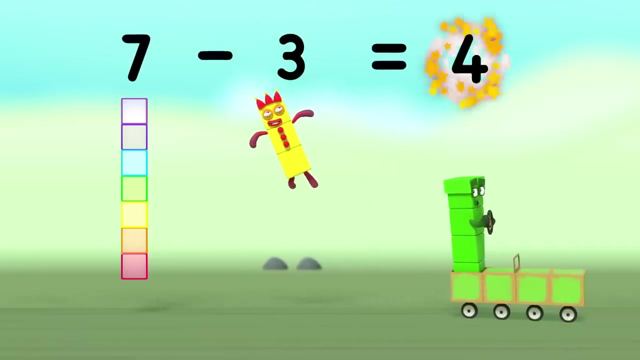 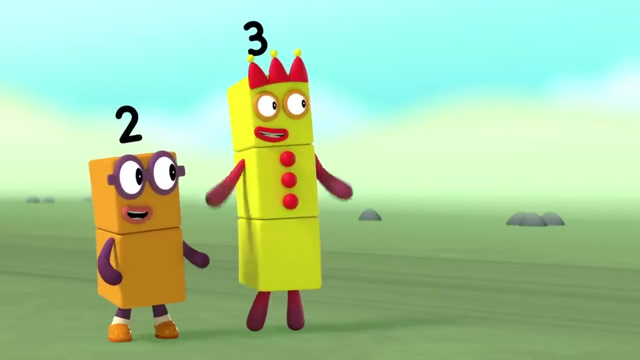 Phew, that was ducky. Seven Minus three Equals four. Four wheel drive: Yay, Yay, Yay, Yay Woohoo. Yay, Yay, Yay, Yay Yay. 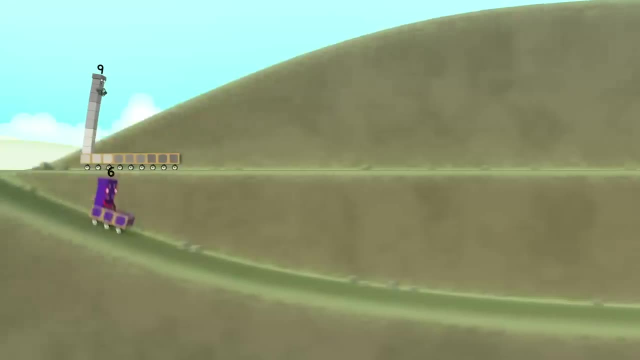 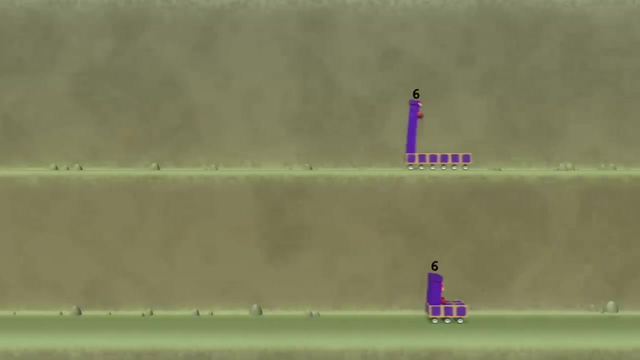 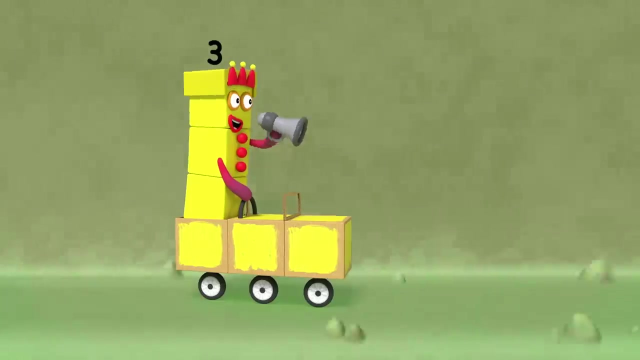 Yay, Six has caught up with nine as they enter the double dipper. Mind that dip: Nine minus three equals six, And the double dips Six minus three equals three. And what a cloche for nine. Six. I'm starting to get fine there. 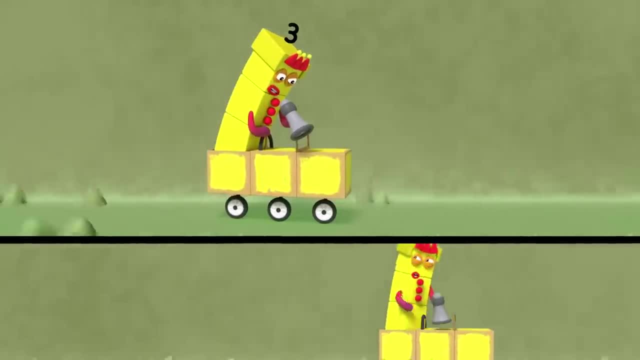 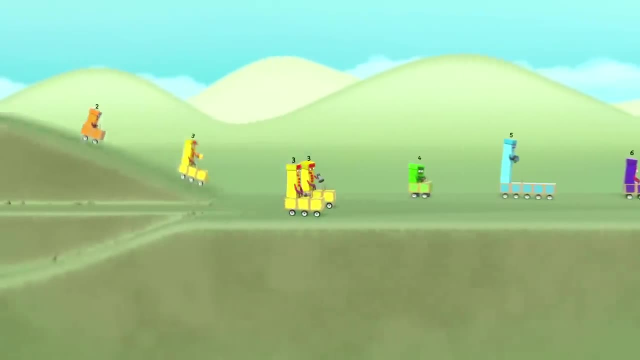 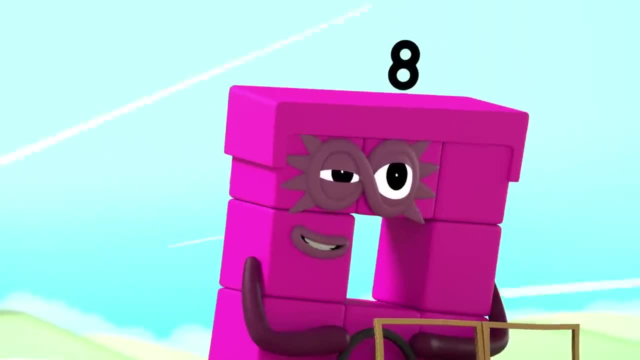 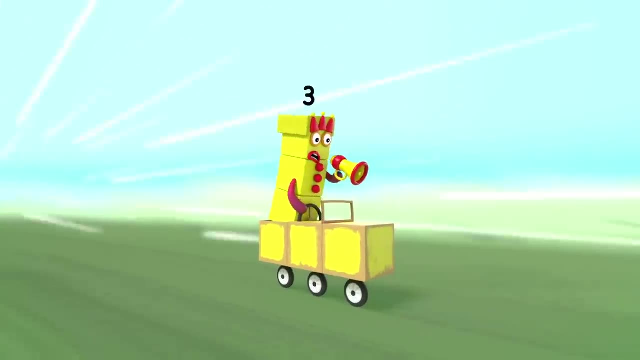 Three, Three equals me Back in action, And with the finish line on the map, is it a gamble? And with the finish line in sight, it's four in the lead. Then I need a breather Octoblock coming through. 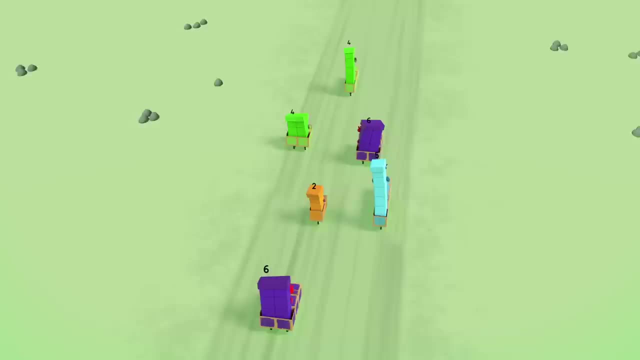 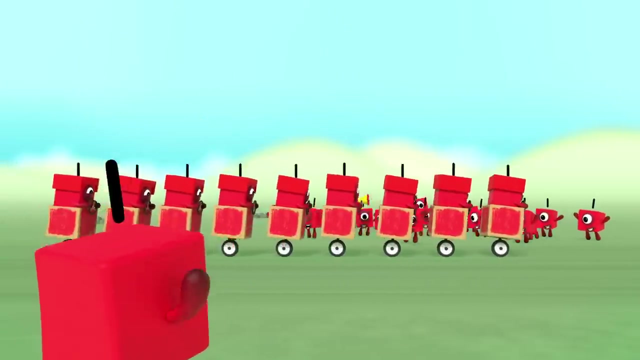 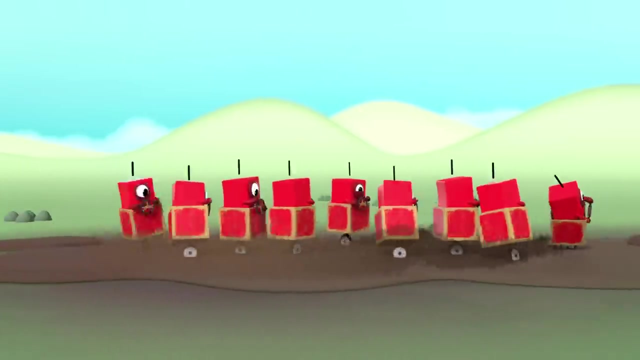 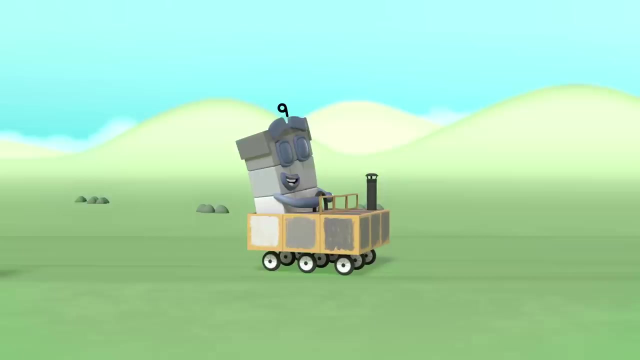 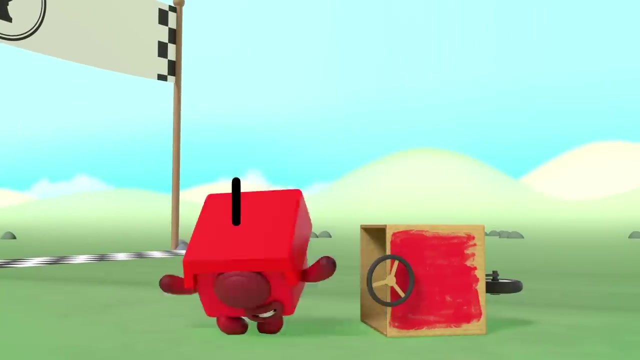 Uh-oh, Uh-oh, And it's one in the lead, followed by one, But here's one coming up on the inside. Nine ones equals Nine. Nice day for it. I'm first. Oh yeah, Ready or not? here I come. 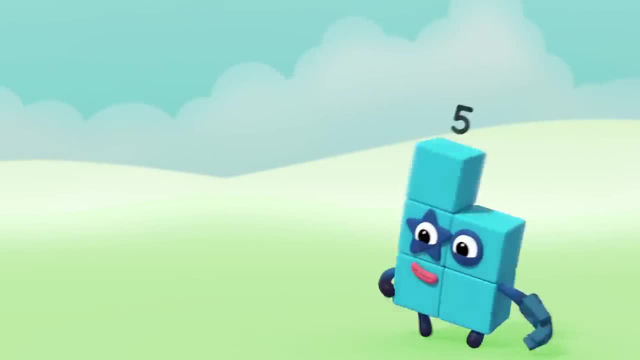 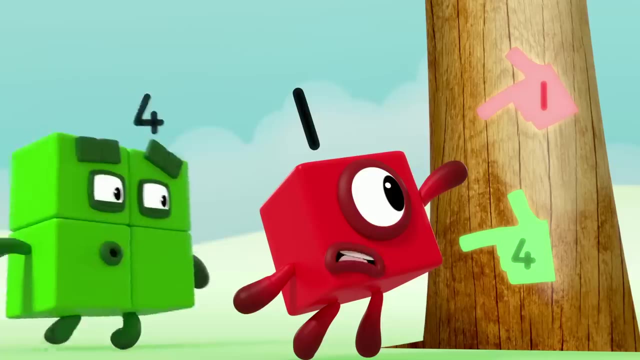 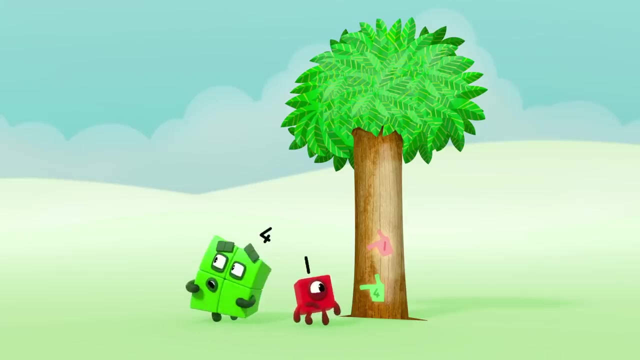 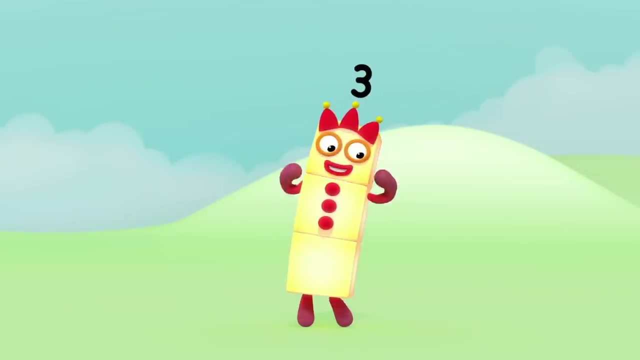 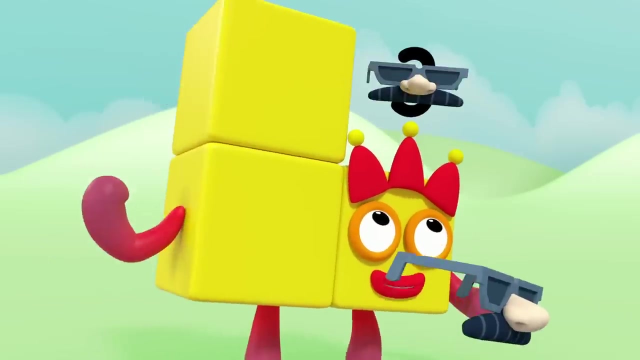 Find you four, find you one. Five minus one Equals four. Look Five, said she'd point us out. Five was right here. How I am. three master of disguise. Shh Ready or not, Ready or not?